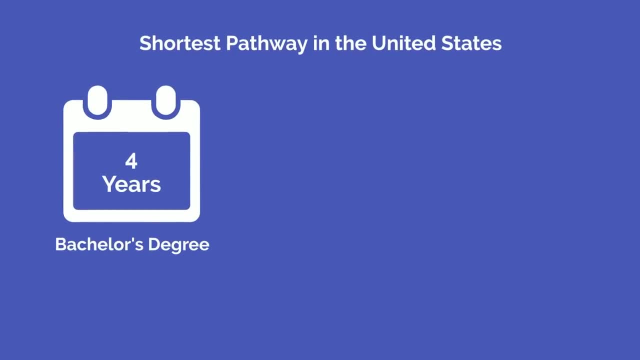 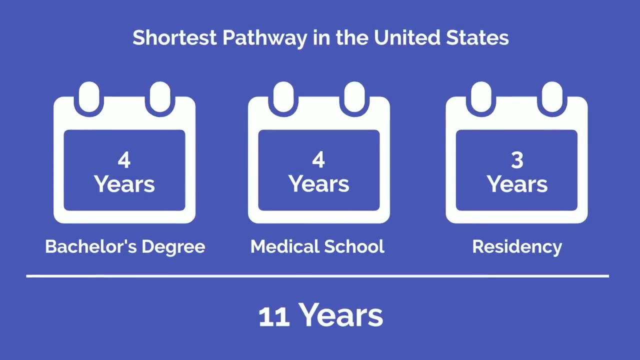 specialty. If we do some simple calculations, the shortest amount of time it would take to become a physician in the United States after high school is around 11 years. That's four years to get your bachelor's degree, plus four years of medical school and three years of residency. 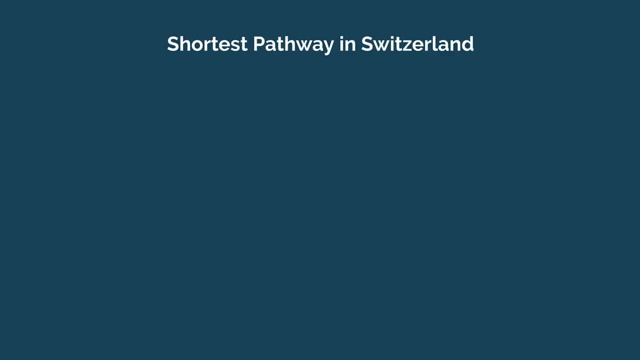 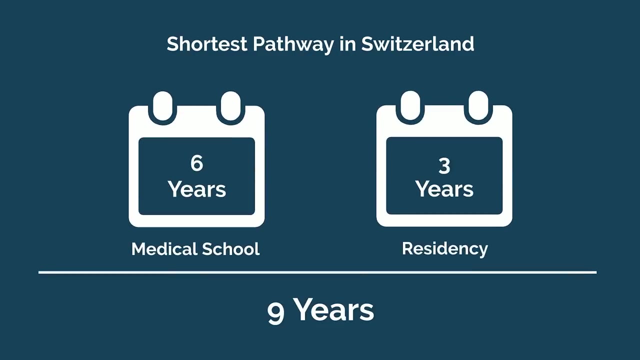 In contrast, the shortest pathway to becoming a physician in many European countries, such as Switzerland, for example, would be six years of medical school, followed by three years of residency, for a total of nine years. Medical school admissions in the US are also highly competitive, which often adds additional years to the already long training process. 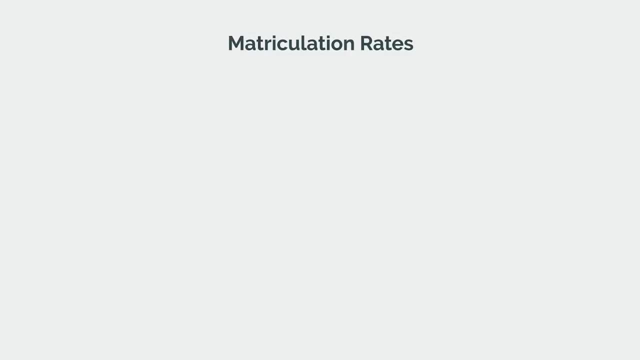 According to data from the AAMC, AACOM and TMDSAS, in any given year, only around 36% of applicants to US MD and DO schools matriculate and only around 25% of applicants to Texas medical schools. 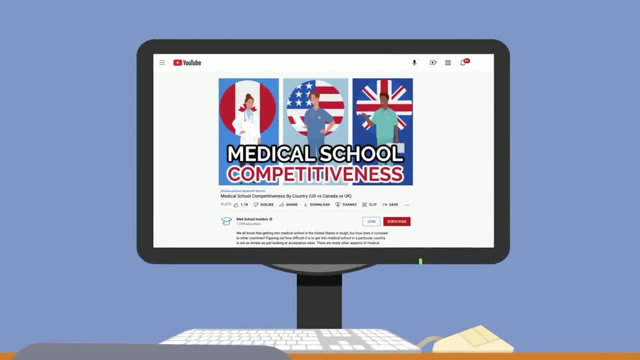 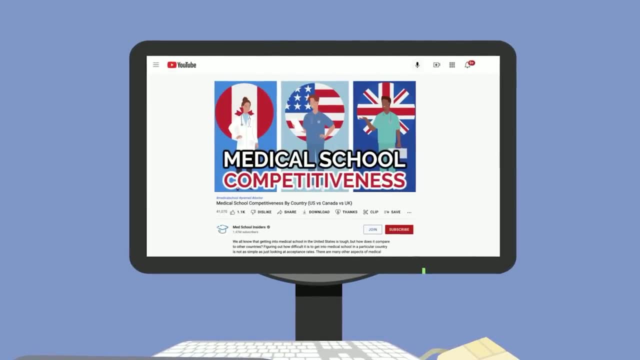 matriculate. Although there are some countries where it is more competitive to become a doctor than in the US, which we discuss in our Medical School Competitiveness by Country video, it is not uncommon for US pre-meds to apply to medical school multiple times before getting. 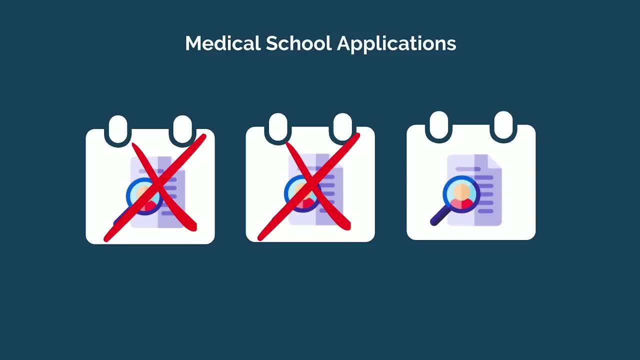 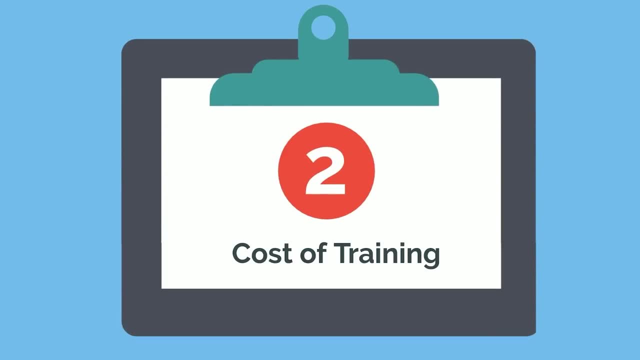 accepted. This is not uncommon for medical schools to apply to medical school multiple times before getting accepted. Because medical school applications occur once per year. each unsuccessful application cycle adds an additional year to the already lengthy training process. Next is the exorbitant cost of medical training, Although physicians in the US earn higher salaries. 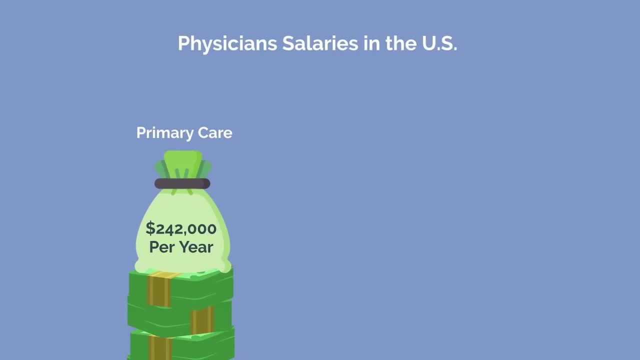 on average than their European counterparts, at around $242,000 per year for primary care physicians and $344,000 per year for specialists. the cost of becoming a physician in the US is also significantly higher. As of 2022,, the average cost of medical school tuition in the United States is: 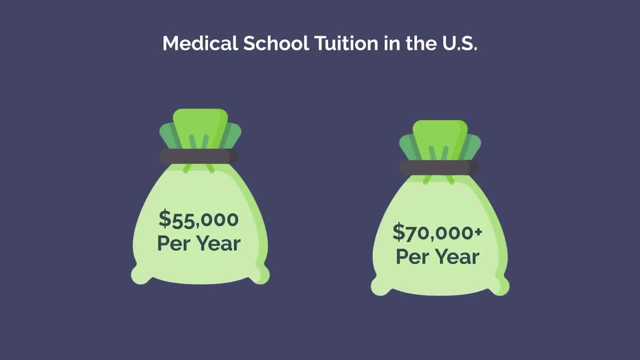 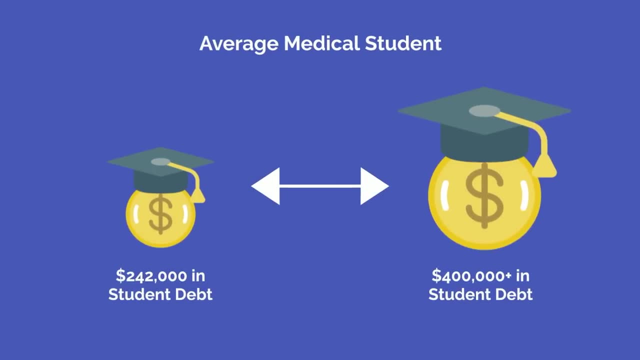 approximately $55,000 per year, with some schools charging in excess of $70,000 per year at the upper end. It's no surprise, then, that the average medical student graduates with around $242,000 of student loan debt, with some students having in excess of $400,000 in student debt between tuition. 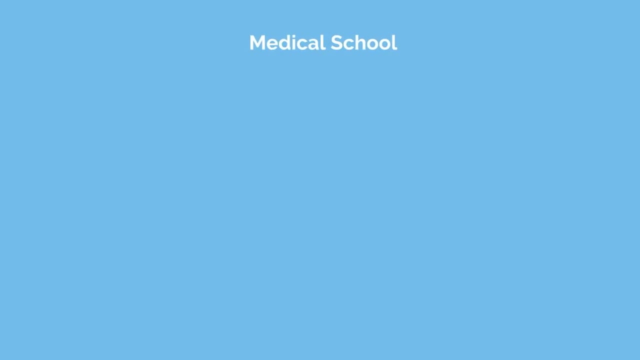 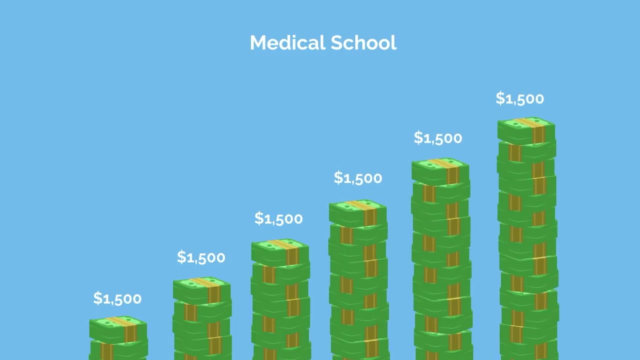 and living costs over four years of medical school. It's only getting more expensive, too, as the average cost of medical school rises by approximately $1,500 each year, Although there are more pre-meds than there are medical school spots, as demonstrated by the roughly 36% of the 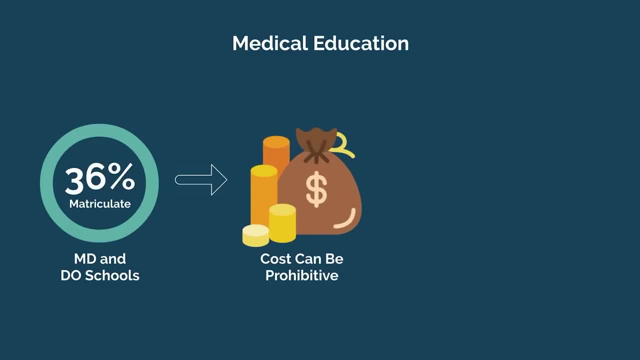 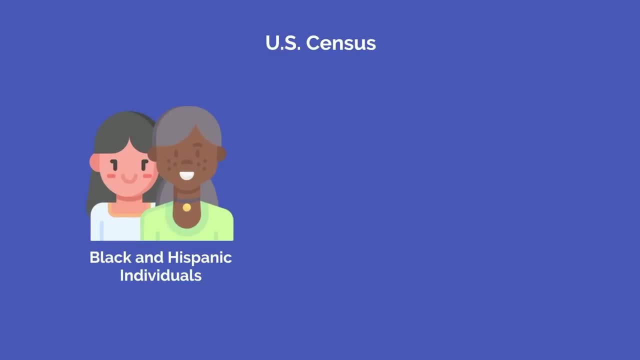 population. the cost of medical education can be prohibitive for many students, particularly minority students and those from lower socioeconomic backgrounds. According to the US Census, black and Hispanic individuals are between one and a half to two times more likely to experience poverty than white or Asian individuals. As such, 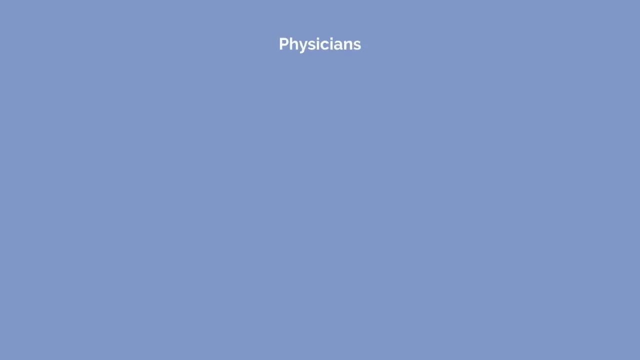 many of these students may be dissuaded from pursuing medicine due to the high cost of medical education. This is an important factor to consider, as research has shown that physicians that come from poor or minority backgrounds are more likely to practice in underserved communities where the 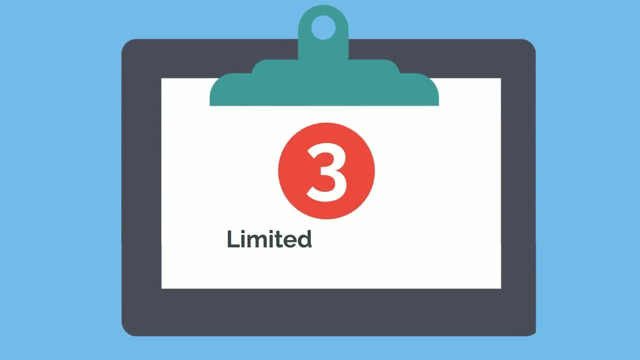 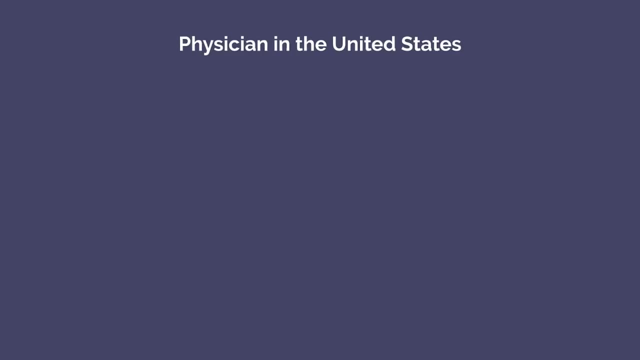 need for physicians is the greatest, Perhaps the largest. factor limiting our ability to produce more physicians, however, is the limited number of residency positions offered each year. To practice medicine as a physician in the United States, you must complete three to seven years of residency training after medical school. The issue is that there are more medical 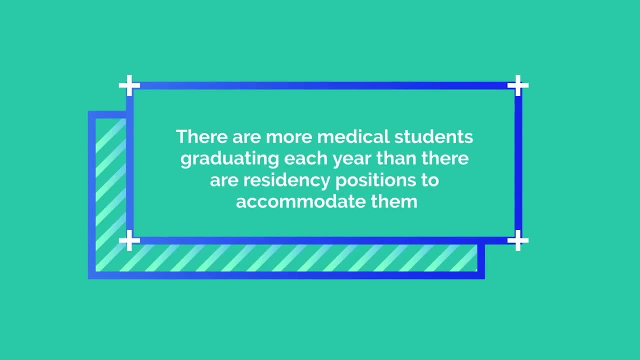 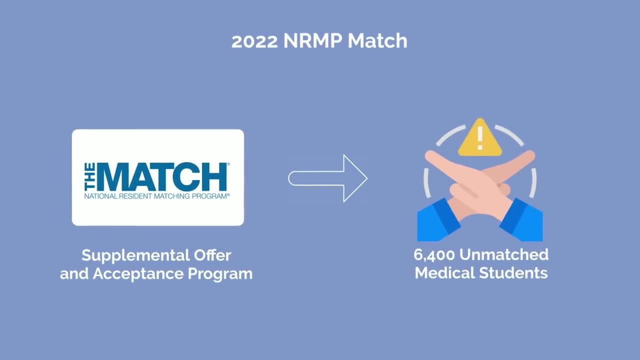 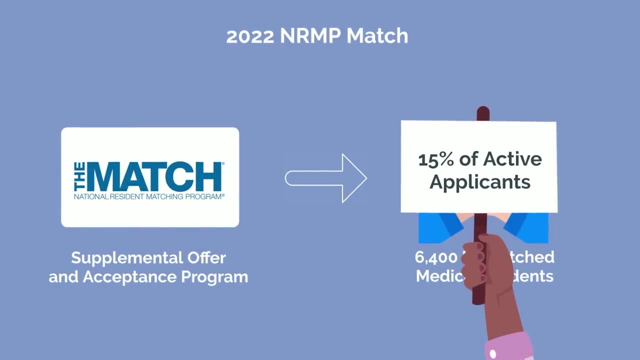 students graduating each year than there are residency positions to accommodate them. During the most recent 2022 NRMP match, there were approximately 6,400 medical students that applied for residency. that went unmatched, even after the supplemental offer and exchange acceptance program or SOAP. That's approximately 15% of the total number of active applicants in 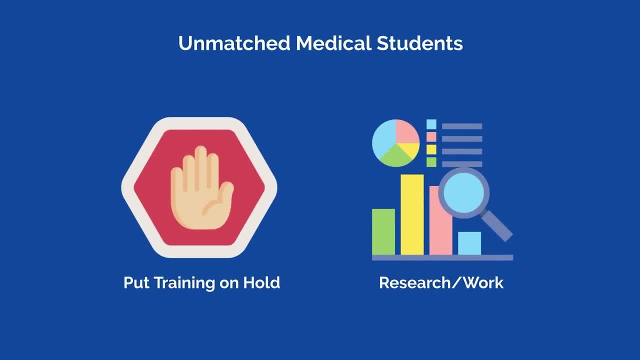 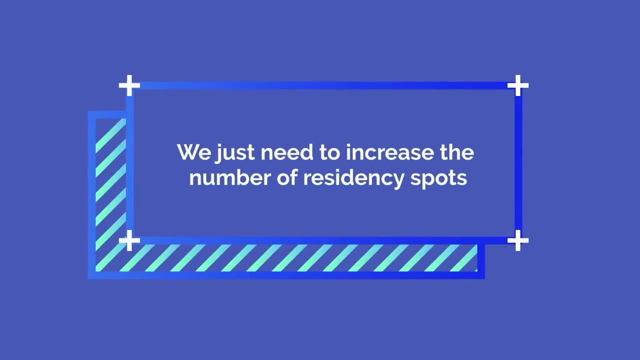 2022.. These students will have to put their training on hold for a year and do research or some other job while they strengthen their application for the following cycle. There's a simple solution, then: We just need to increase the number of residency spots Easy. 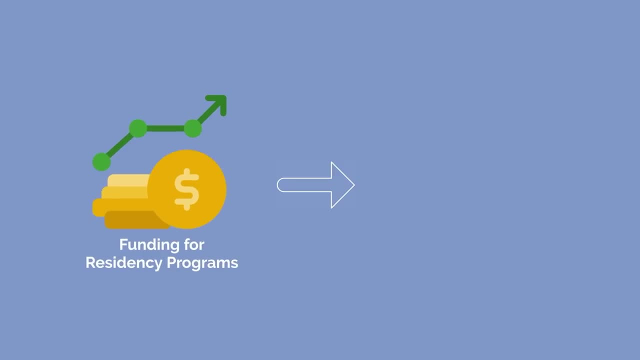 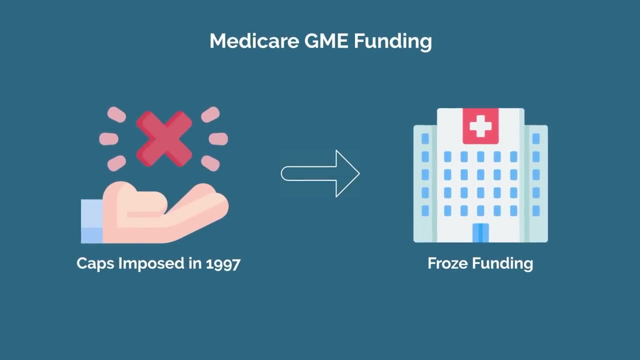 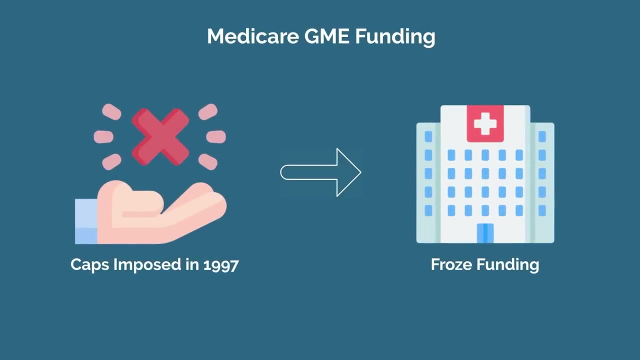 right, Not quite. The majority of funding for residency programs comes from Medicare. The problem with this is that there were certain caps on Medicare GME funding imposed in 1997, which have largely frozen in place the facilities eligible to receive funding. This in turn has greatly hindered our ability to open new residency programs. 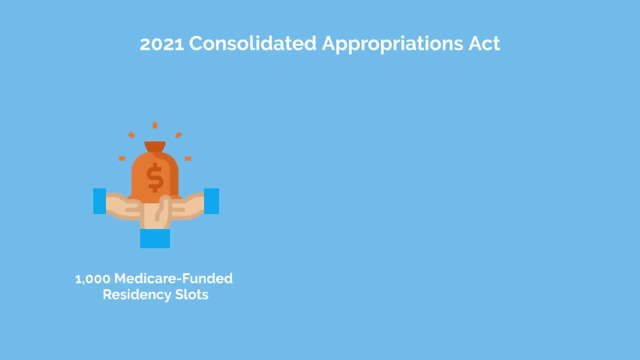 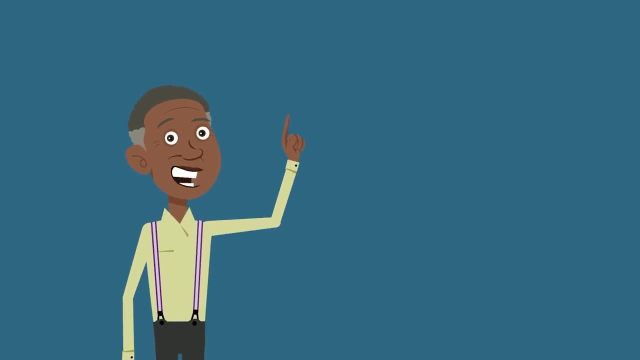 This is slowly changing with the recent 2021 Consolidated Appropriations Act, which will have Medicare provide an additional 1,000 funded slots over five years, starting in 2023.. However, many are concerned that the existing system still does a poor job at creating. 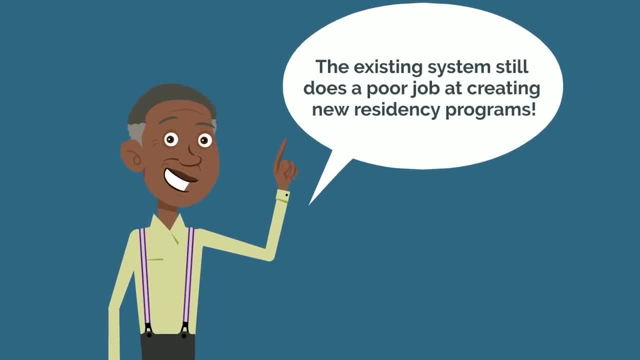 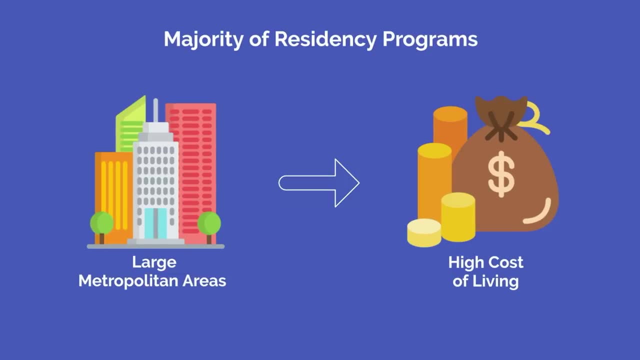 new residency programs for a variety of other reasons. To start, the majority of residency programs are in large metropolitan areas where the cost of living is high. As such, each dollar spent on funding residency programs doesn't go as far as it would if these programs were in areas with lower costs of living. It would make much more. 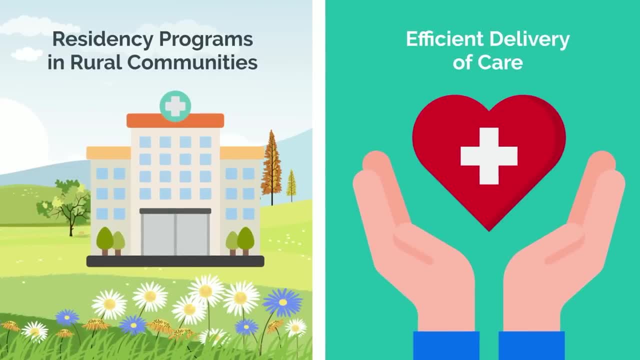 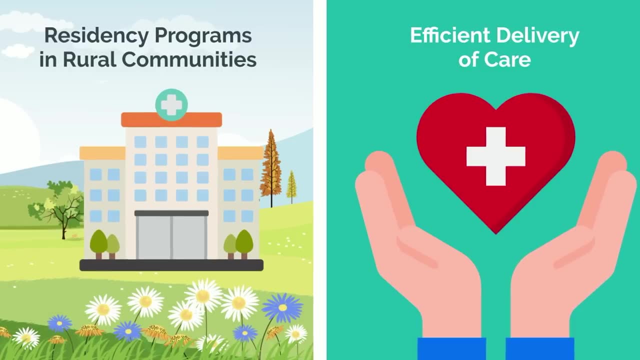 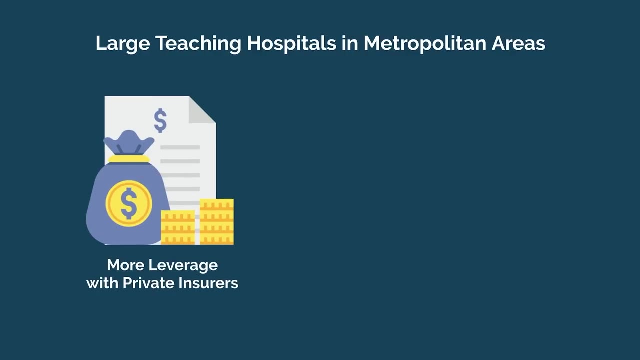 sense to establish residency programs in rural communities, where care could be delivered more efficiently to the patients that need it most. Despite this, residency programs are much more abundant in large metropolitan areas compared to rural areas. This is largely a consequence of large teaching hospitals in metropolitan areas having more leverage with private insurers. to 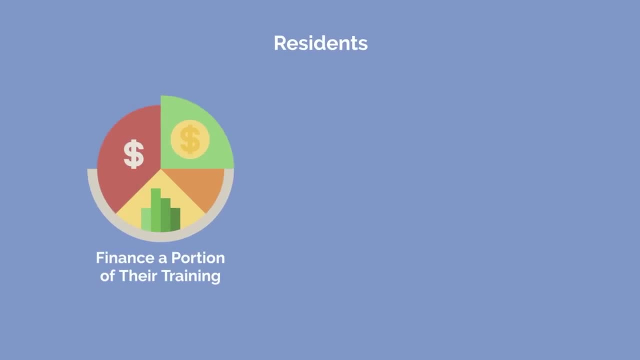 gain higher reimbursement rates for residents. Residents implicitly finance a portion of their training through their contributions to patient care. As such, there is often less financial risk to hospitals starting residency programs in these big metropolitan areas, as they often receive higher reimbursement rates for services provided. 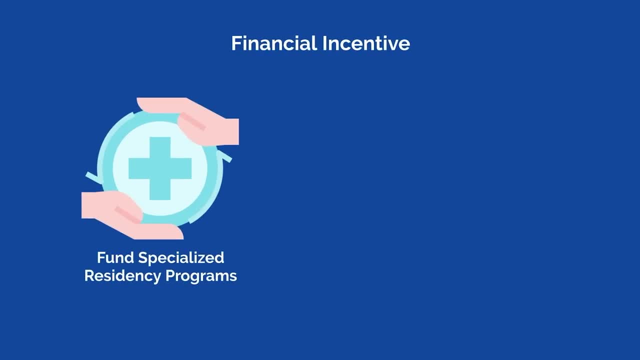 by residents. In addition, there is often more financial incentive to fund specialized residency programs as opposed to primary care specialties, despite the latter being in greater need, as reimbursement rates for specialists tend to be much higher. For these reasons, just throwing more money at the problem of the limited number of residency positions. 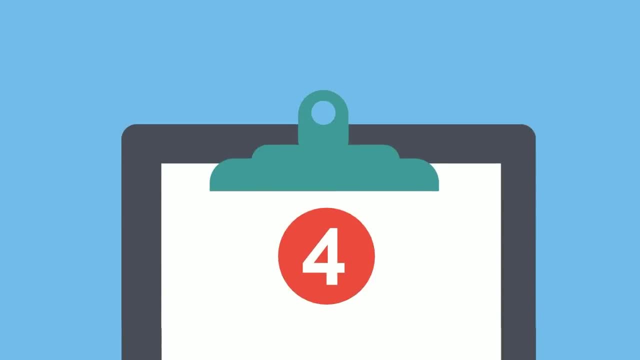 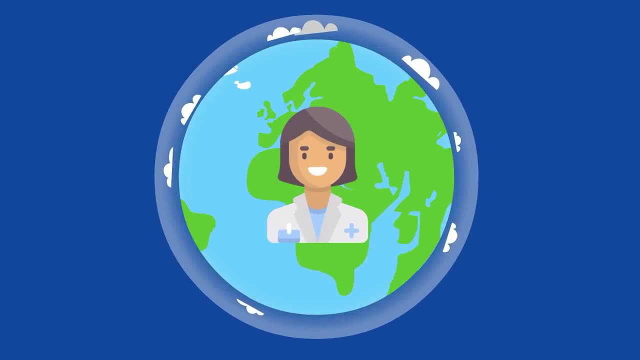 may not be sufficient. That being said, increasing the number of physicians trained in the US is only one solution to the physician shortage. Another solution is to import physicians from other countries to practice in the United States. The issue is that there is a lot of red tape, that 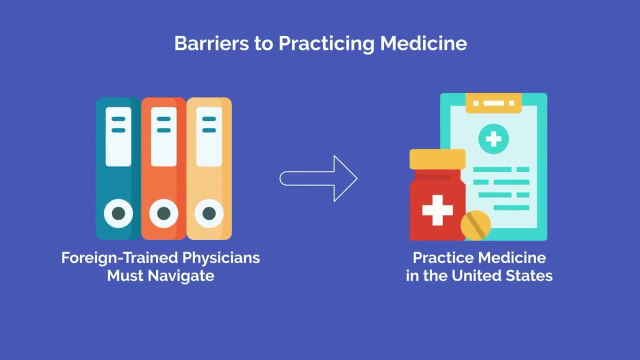 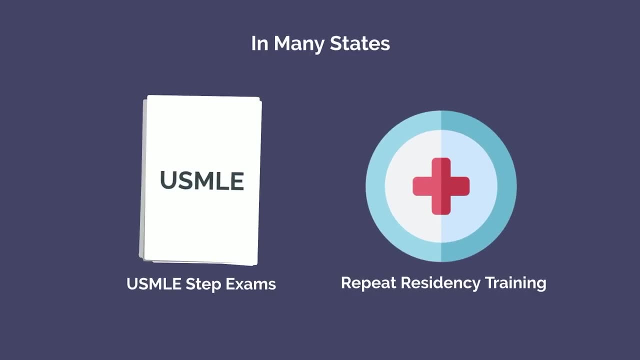 foreign-trained physicians must navigate in order to practice medicine in the United States. In many states, foreign-trained physicians are required to take the USMLE step exams and repeat residency training, which can be a huge barrier to entry for physicians who have been practicing for many. 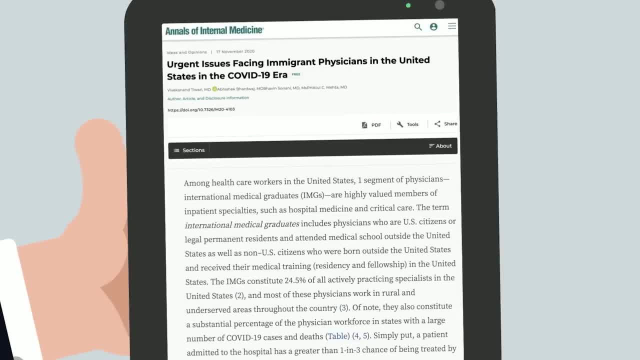 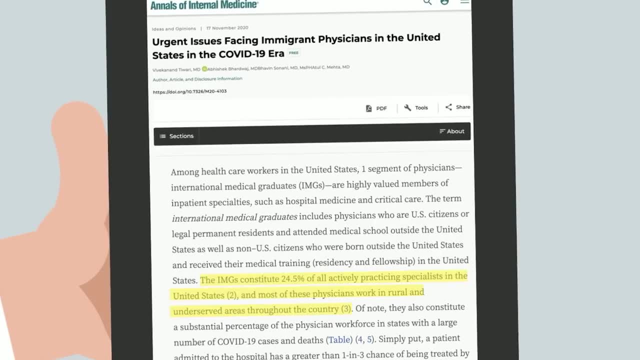 years and are well-established in their specialty. In a 2020 article in the Annals of Internal Medicine, international medical graduates, or IMGs, constitute about 25% of all actively participating specialists in the United States and most work in rural and underserved areas throughout the country. This may sound like a 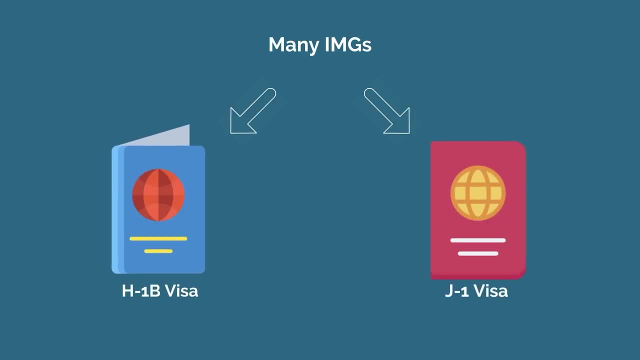 lot. However, many IMGs are only here on temporary H-1B and J-1 visas while completing residency training. IMGs that hold a J-1 visa are required to return to their home country for two years after completing their residency or finish a three-year waiver position in an underserved 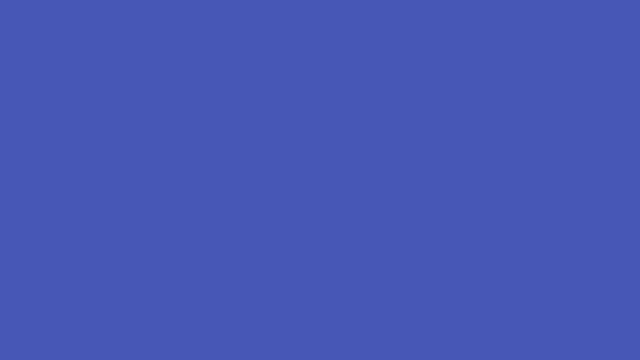 area before they can apply for a residency. This is a huge barrier to entry into the US and is a huge barrier to entry into the United States. IMGs holding an H-1B visa may apply for a green card and permanent residence after they complete their residency. That being said, 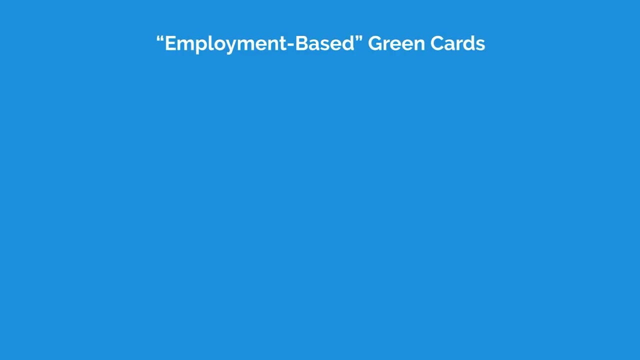 just because they are eligible for a green card does not mean that they will receive one. Green cards issued under the employment-based category, such as for residents, have a total cap of only 140,000 green cards per year, with a fixed cap of 7% allotted to each country. 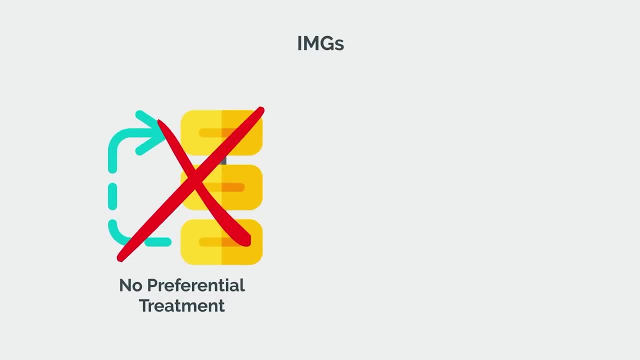 In addition, IMGs do not receive any preferential treatment in obtaining their green card for being a physician And even after receiving a green card, there are more and more of these green cards that have multiple hoops to jump through to practice as a physician permanently in the US. 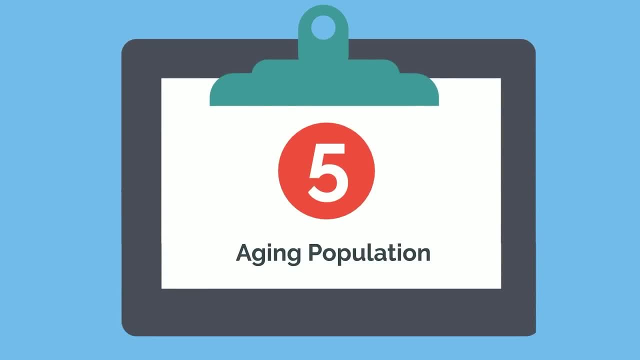 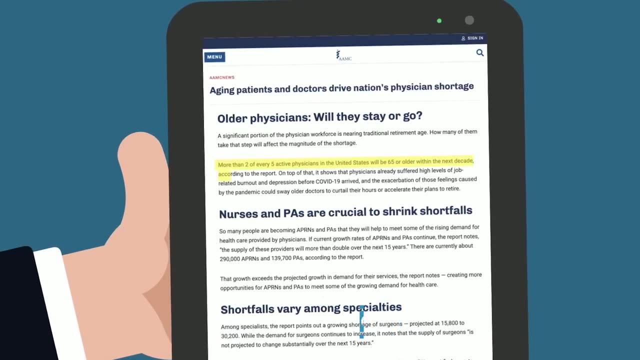 Lastly, a growing and aging population combined with an aging workforce of doctors nearing retirement has further exacerbated the issue of physician shortages. The AAMC estimates that within the next decade, more than two out of every five practicing physicians will be over the age of. 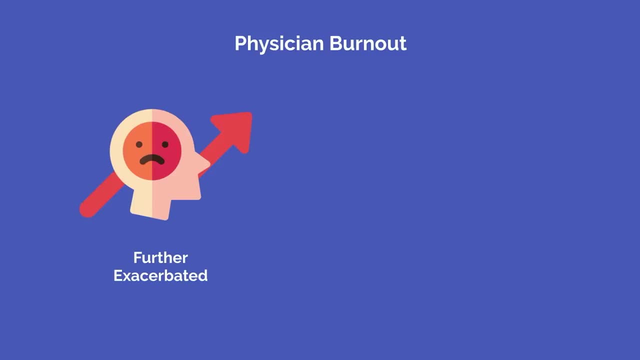 65.. In addition, physician burnout is a huge issue within medicine, which has been further exacerbated over the past few years as a result of the COVID-19 pandemic. These issues may lead some physicians to decrease their hours or even lose their ability to practice. So if you're 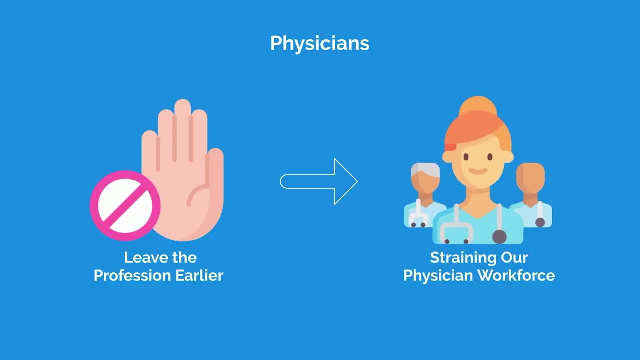 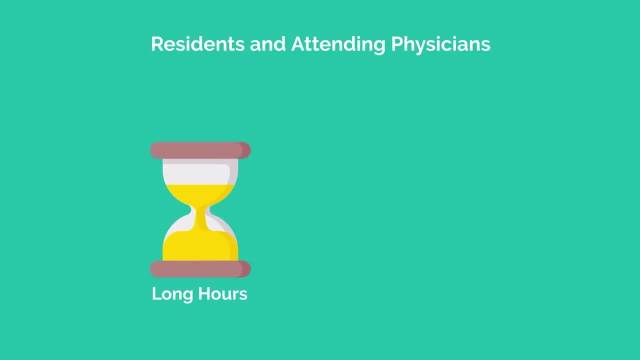 interested in learning more about these issues, you can subscribe to our YouTube channel by clicking on the little bell on the top right of this video. This is another big reason why we need to take steps toward increasing the number of physicians in the United States. The long hours and difficult schedules that resident physicians and attendings 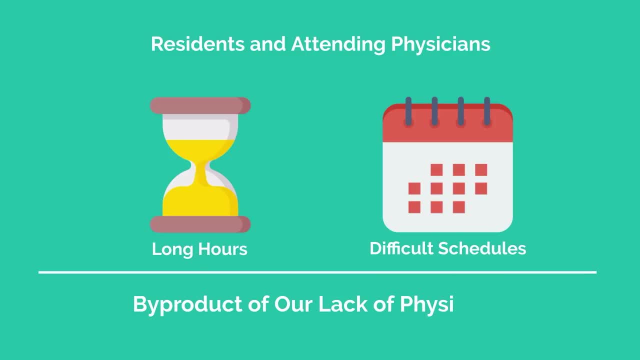 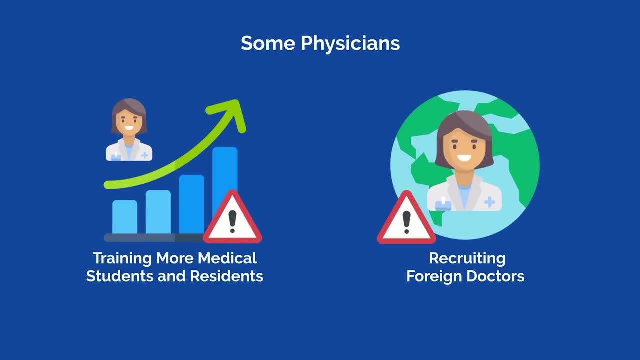 work are not a matter of necessity, but rather a byproduct of our lack of physicians. Some physicians oppose training more medical students and residents or recruiting foreign doctors, as they fear it will decrease their salaries. Although this is a reasonable concern, having more doctors is likely to make life better for US doctors. 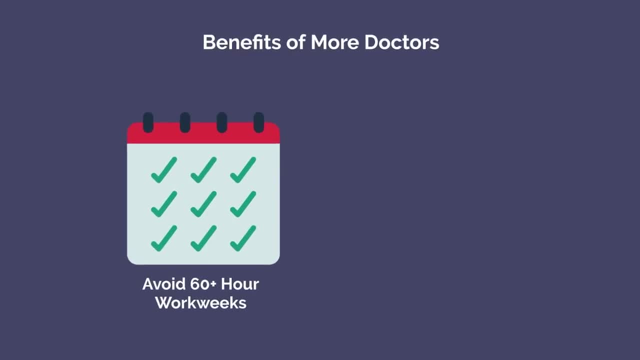 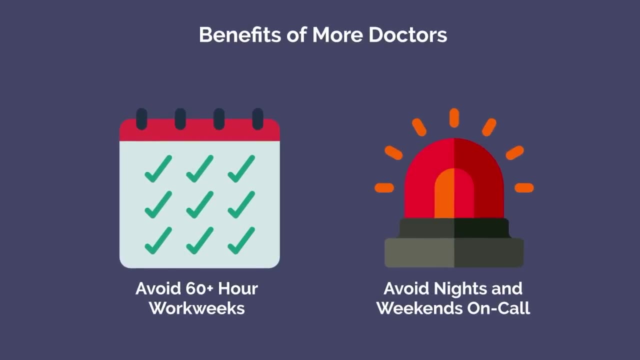 By sacrificing a bit of pay, they may be able to avoid 60 plus hour work weeks and having to spend nights and weekends on call. That being said, the one area that we need to remain cautious about as we take steps to address the physician shortage is the rising cost. 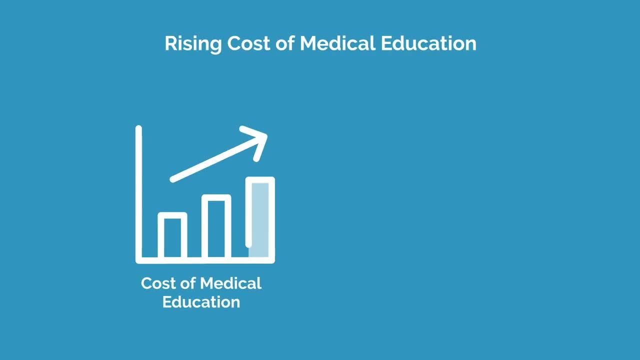 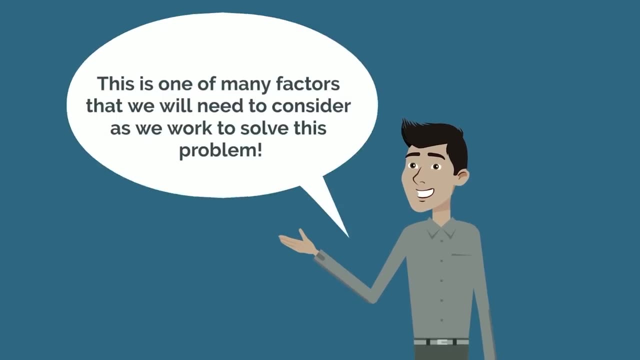 of medical education. If the cost of medical education continues to increase at the current rate and salaries for physicians start to decrease, we may end up with a generation of physicians with massive debt that they struggle to pay back. This is one of many factors that we will need to consider as we work to solve this problem. As you can see, 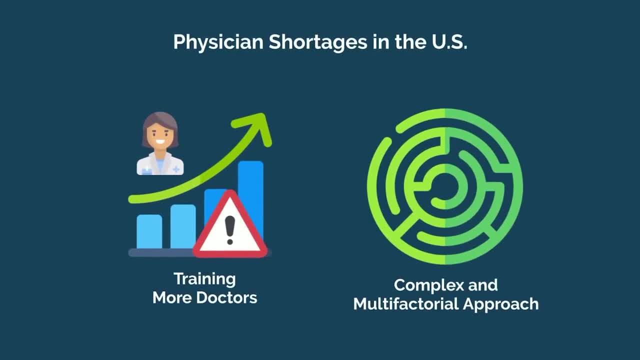 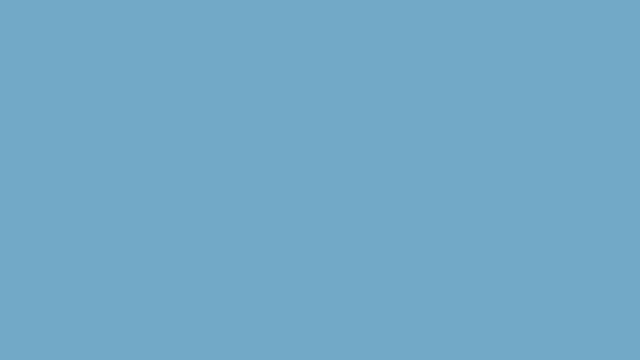 the issue of physician shortages in the US is not just a matter of training more doctors. It is a complex issue with many different factors that will require an equally complex and multifactorial approach. We need leaders and policy makers to take a good, hard look. 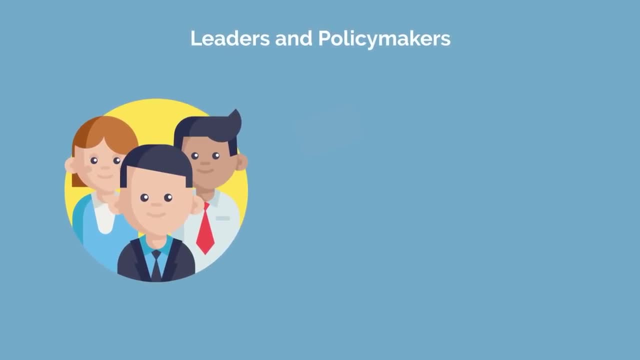 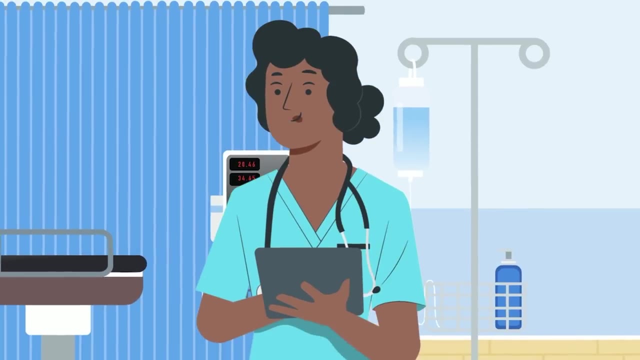 at the state of medical education and physicians in the US and start making steps toward addressing issues like the rising cost of medical education, physician burnout and the lack of residency positions. Only then will we be able to meet the growing demand for physicians in the United States. If you enjoyed this video, I know you love my free. 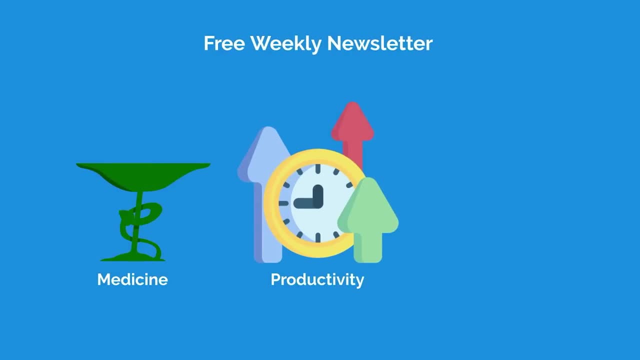 weekly newsletter where we talk about all the things you need to know about medical education in the US and where we cover these and similar topics in medicine productivity and study strategies. You'll also get access to the best study music with my Study With: